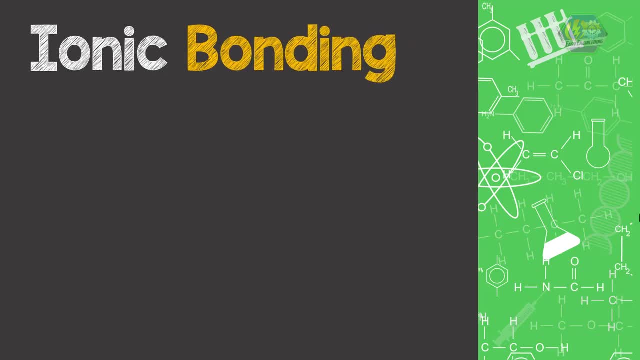 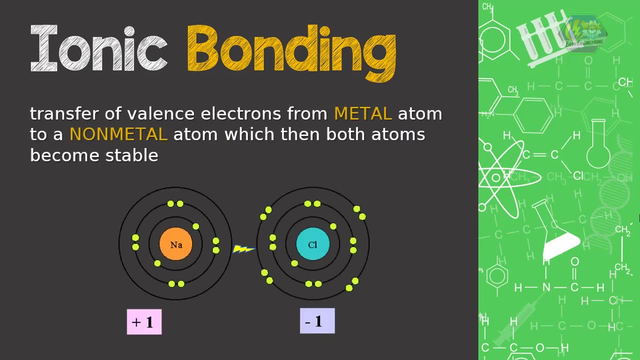 To start with ionic bonding. Ionic bonding occurs between metal and non-metal atoms. It involves a transfer of valence electrons from metal atom to non-metal atom, which then both atoms become stable. Each atom bearing a positive or negative charge is called ion. 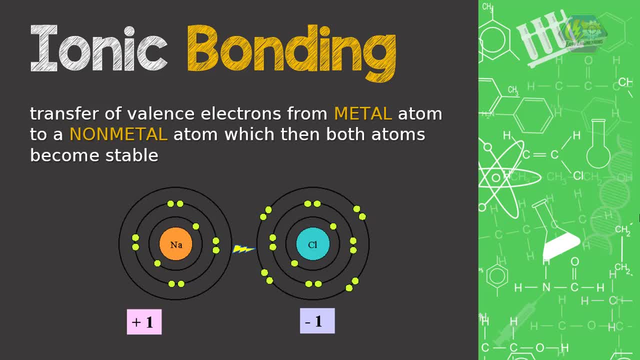 Because of the transfer of electrons, the metal atom have a net positive charge and the non-metal atom have a net negative charge. The ion that carries a positive charge is called cation, While the ion that carries a negative charge is called anion. 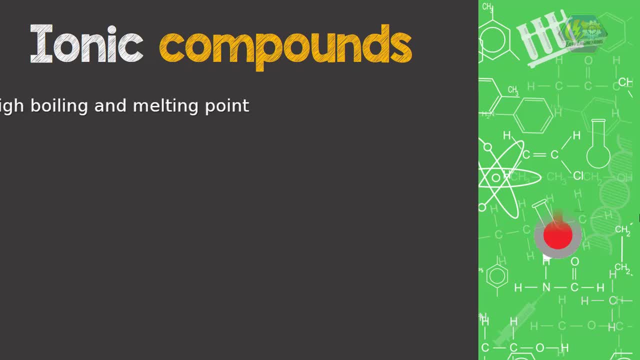 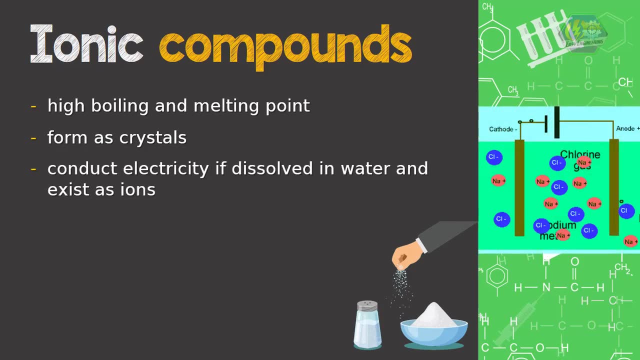 Basically ionic compounds have high boiling and melting points and mostly they form as crystals. They can conduct electricity if they are dissolved in water and exist as ions. Lastly, they are brittle and easily broken down into small pieces. The second type of bonding- 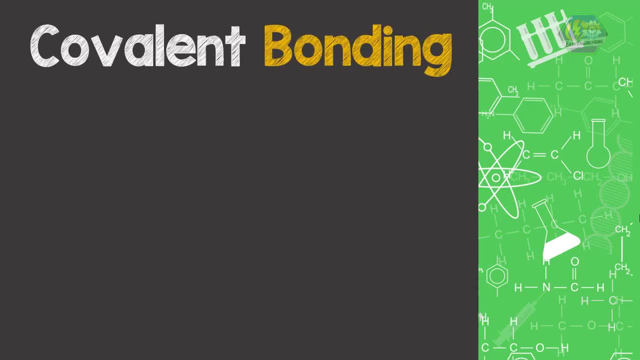 The covalent bonding. Covalent bonding occurs between non-metal and non-metal atoms. It involves a sharing of valence electrons between non-metal atoms for them to become stable. Hydrogen oxygen, chlorine and many others exist as diatomic molecules, which means that there are two atoms of hydrogen oxygen and chlorine for them to exist. 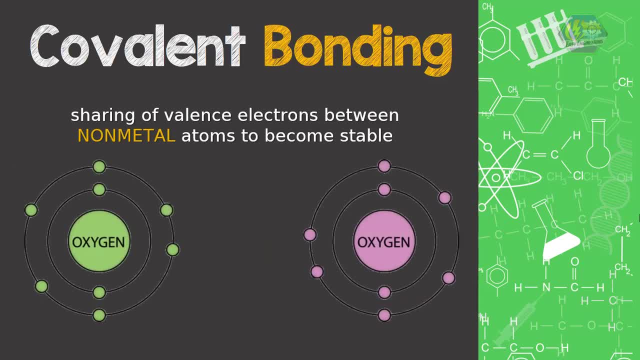 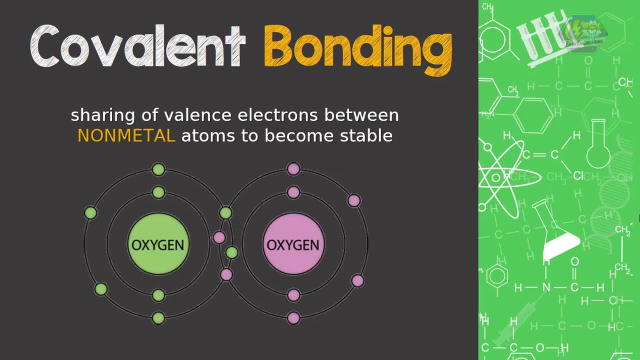 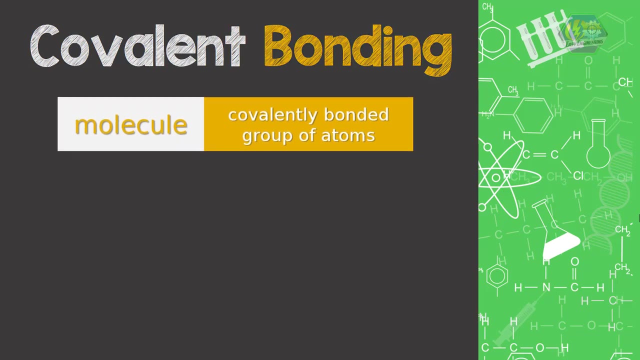 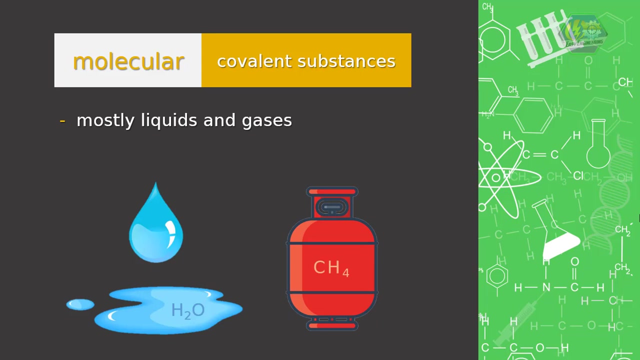 The oxygen atom is covalently bonded with another atom, The same with other diatomic molecules. In chemistry, the term molecule refers to the covalently bonded groups of atoms. Molecular covalent substances are mostly liquid and gases, because the molecules have more freedom to move within the substance. 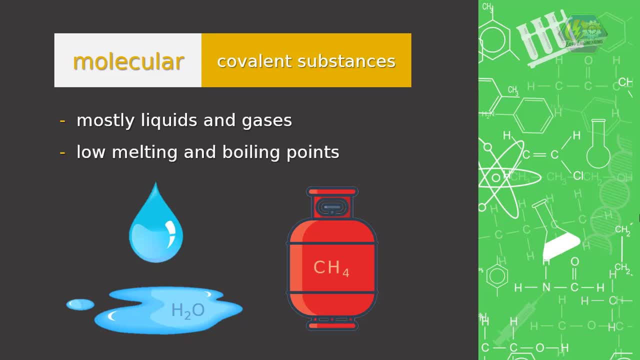 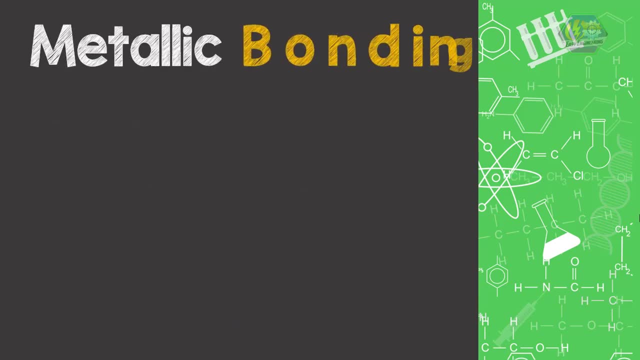 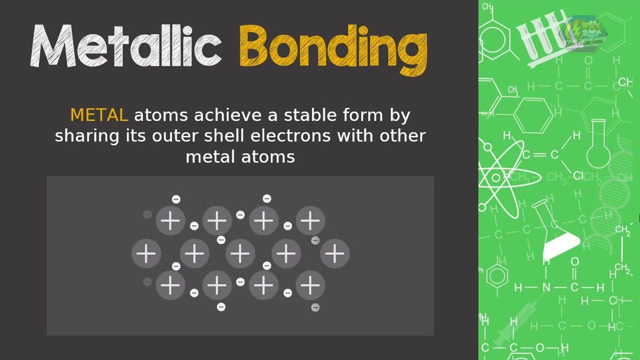 Also, covalent compounds have low melting points and boiling points. The third type of bonding: Metallic bonding. It occurs between metal atoms. Metal atoms achieve a stable form by sharing its outer shell electrons with other metal atoms. The valence electrons of each metal atom are not tightly bound in the nucleus.